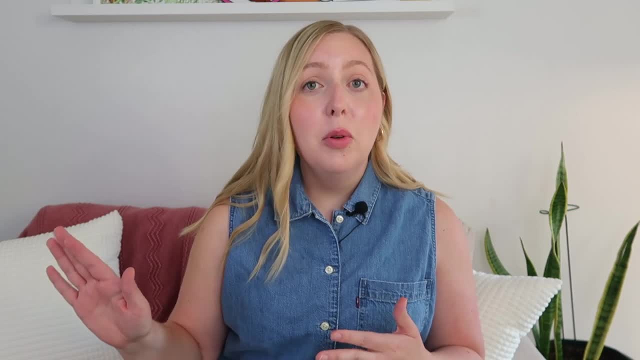 going to get there, We're going to get there, We're going to get there, We're going to get there. Expectations and we know our seating chart. the rest of the year will go so much smoother, rather than kind of skipping over that or trying to speed through it really quickly And just knowing that. 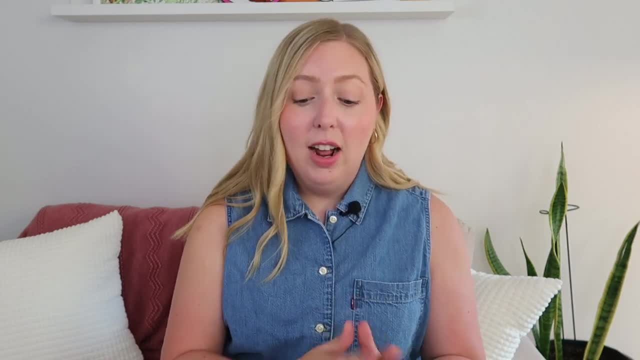 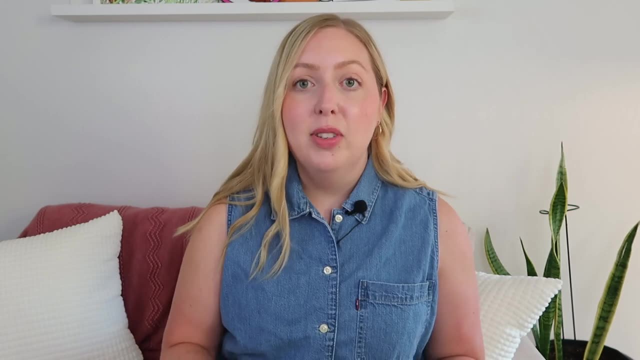 like the first few days are going to be that. So I would say, you know, I have a lot of fun ideas for you guys and I'm excited to share them with you, but also just make sure that you really are going through those rules and procedures, those first few lessons, to really set the expectation for the 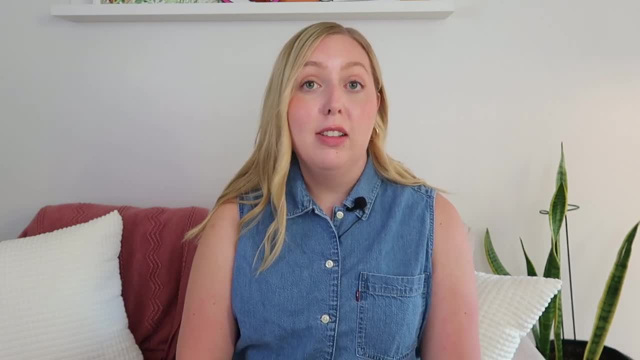 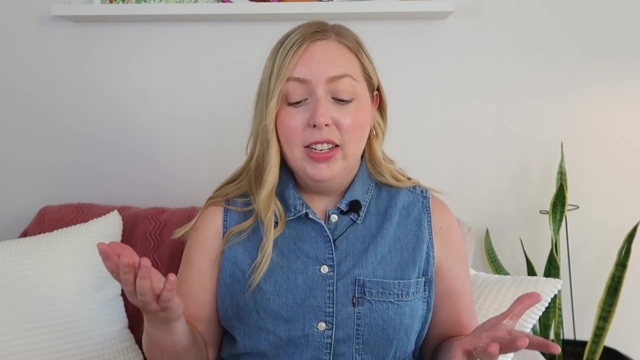 rest of the year. Okay, So upper elementary. I feel like sometimes it's a little tricky on, like what can you do, Um, for that first day to kind of get them engaged and get them excited about music? And so the very 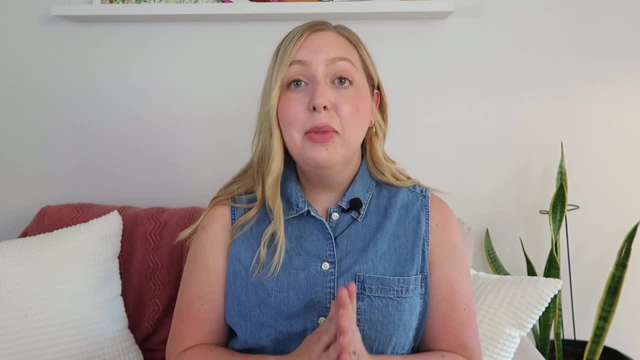 first one I actually did just this year, um about two weeks ago, and it was. it went really well, So it is called musicians move. I talked about it in a vlog. actually I have a first week vlog. 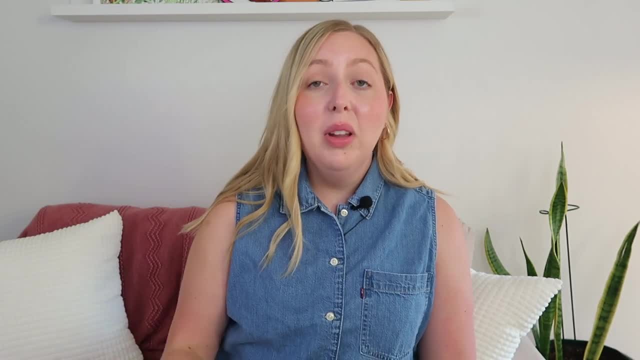 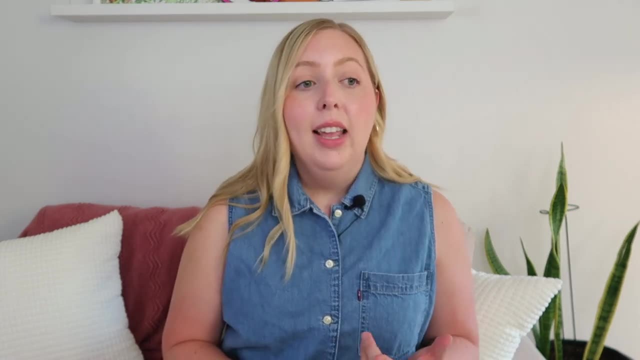 And so I just I'm going to talk about it again because I thought it went really really well. So I think the first day with my upper elementary students, I really like to get to know them musically, Like what's their musical background, And so we played a game called musicians move. 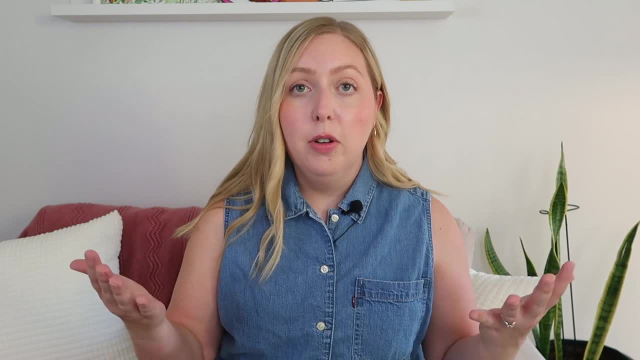 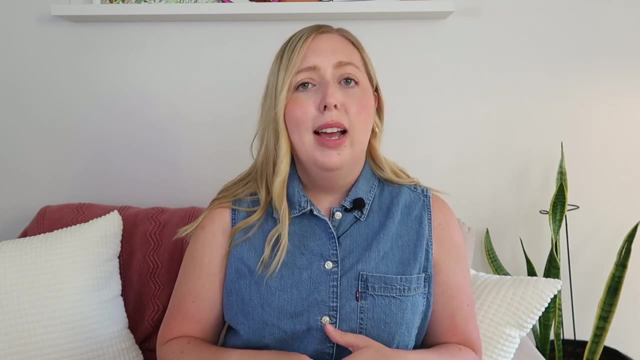 And so how this works is: you are going to have your students in a circle and you can have like a poly dot. You could have a little mini hula hoops. Um, you could have a piece of Velcro on the floor. You could have any. 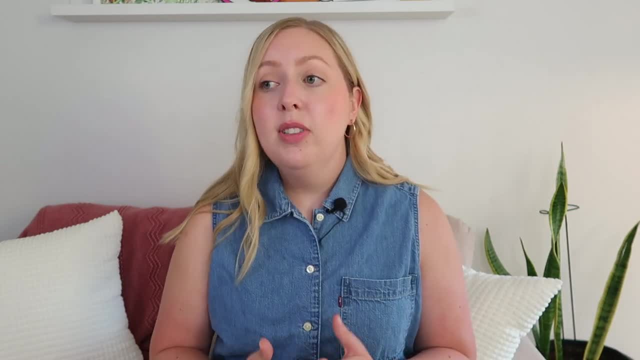 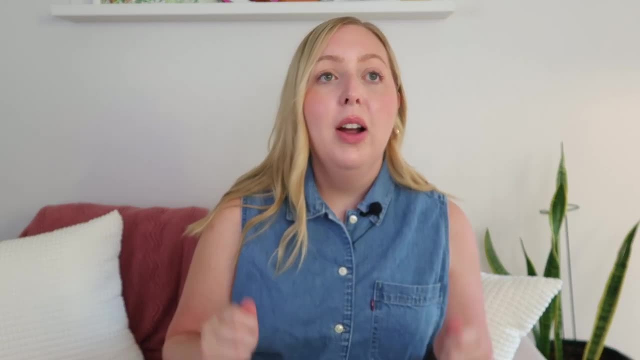 way that you can have a mark. You could have them sit in chairs or stools, but every student is going to sit or stand on their marker. Then you're going to go to the middle and you are going to use these cards, Um, and they're going to have musical statements on them. 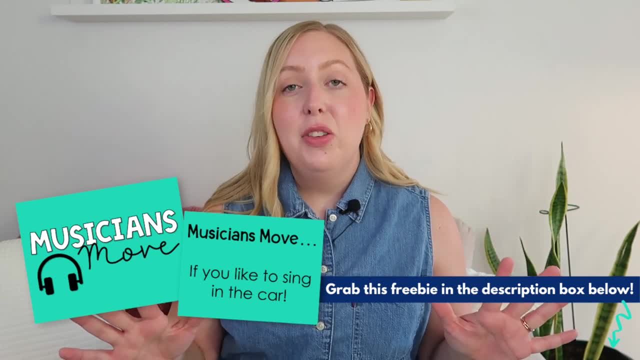 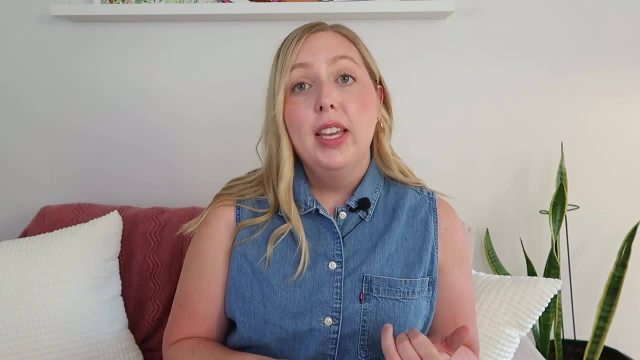 Again, I'll have those linked down below for a freebie for you guys, Um, so that you you can use them in your classroom. So these are going to have statements like I don't know, like an artist that they like move, if you like Ariana Grande. 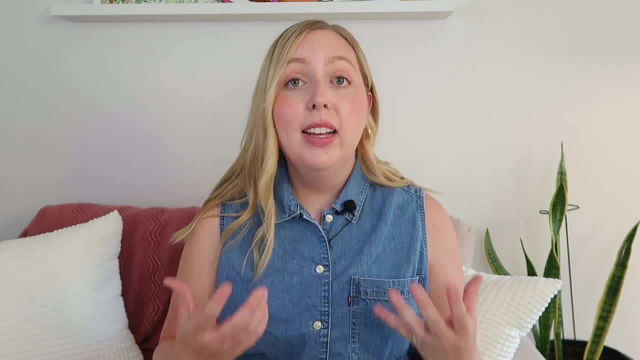 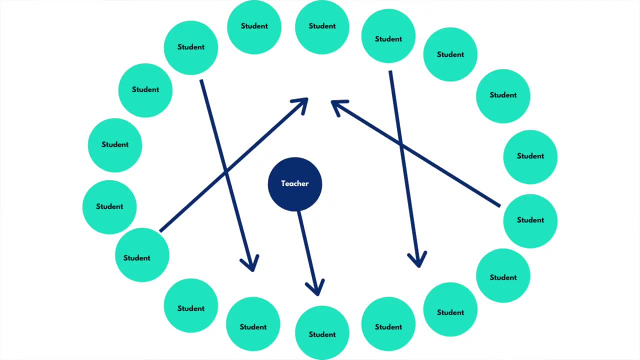 And so I explained. if they agree with that that applies to them and their musical background. then they have to step into the circle and they have to switch and try and find a new hula hoop or whatever the marker is. So they're going to have to find a new place to stand or sit. 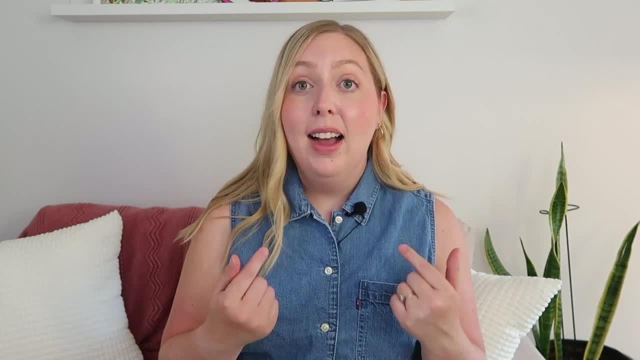 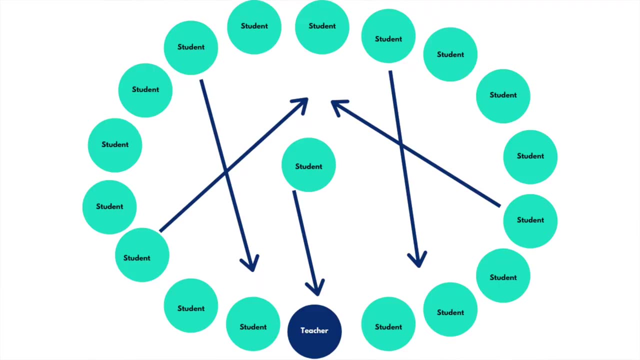 And so they're going to have to switch. Now- hopefully I will be. after I read that First one, I am going to go steal someone's hoop, And so that there is a new person in the middle And I'm going to also take my paper with me, because then I know I've already had a turn. 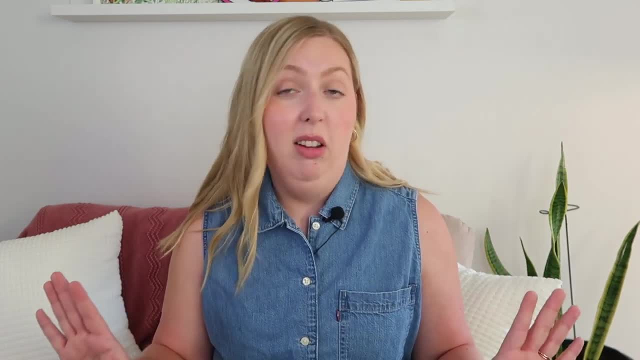 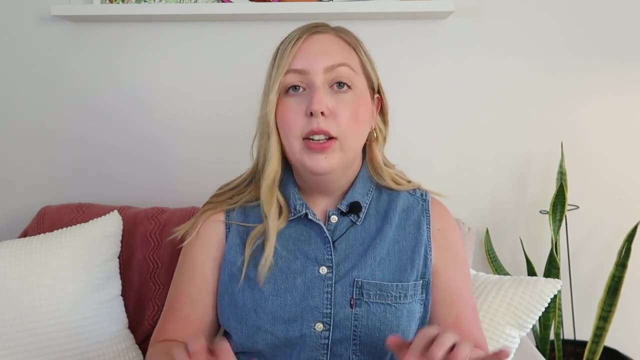 So we play kind of a practice round. I say, okay, let's just pretend everyone loves Ariana Grande And you guys are all going to move and try and switch with someone new. I'm going to steal a hoop, So hopefully there'll be a new person in the middle and don't worry, There's not much pressure. 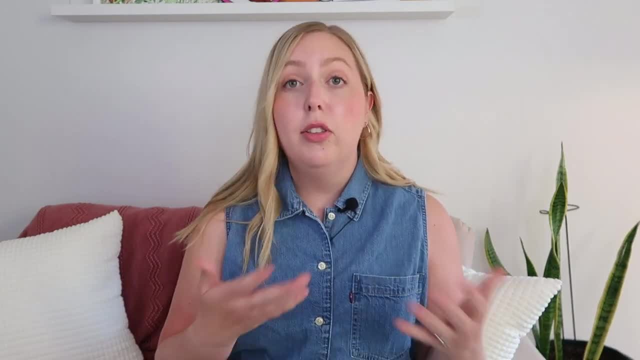 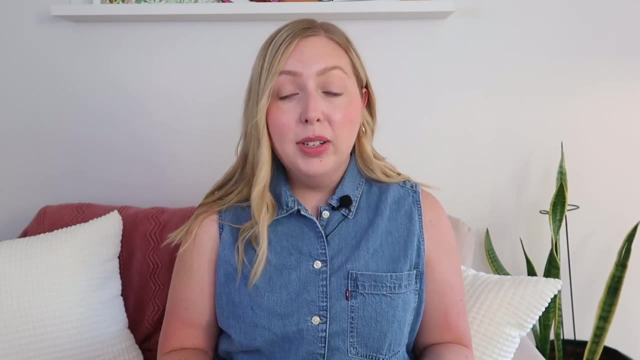 because you don't have to call it the statement. You're just going to read the card, whether you agree with it or not. You're just going to read it for us so that we can switch again, And so we'll do that. And then there'll be a new student in the middle and they have to read a. 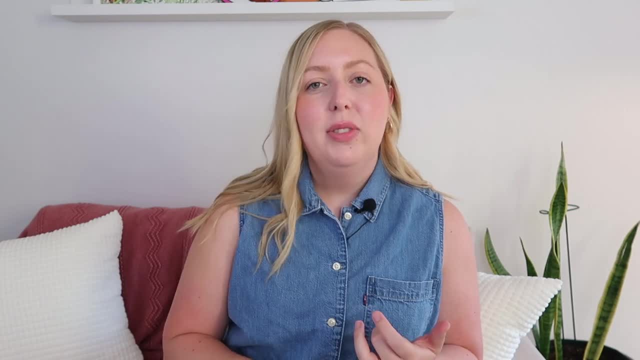 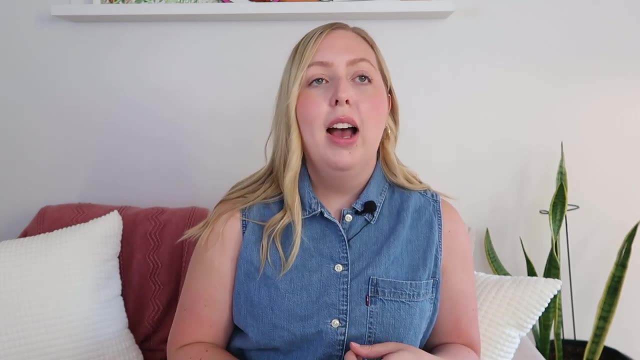 card And I have all kinds of things like if you like to listen to music with screaming in it, AKA screamo move, If you've ever made a music video, if you've ever written a song, if you have a family member that plays an instrument or likes to sing. 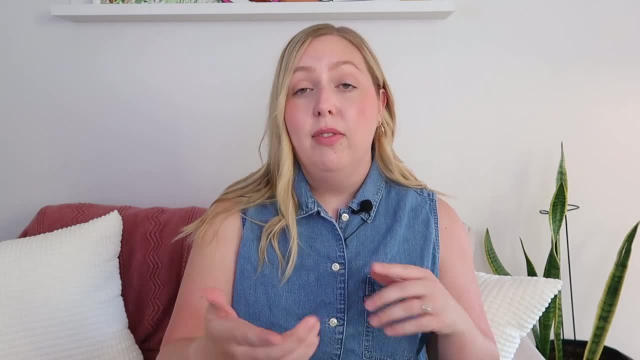 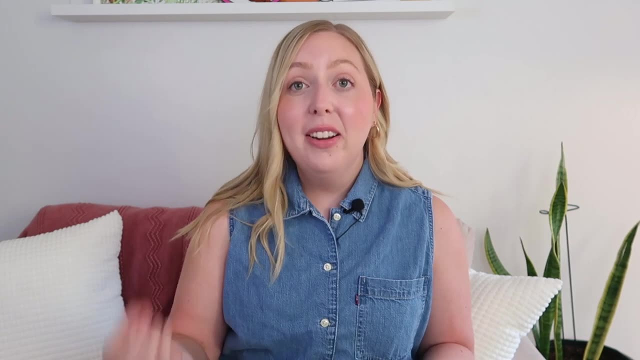 And so it's just kind of getting an idea for students to see connections of their musical backgrounds. It's really interesting to see what they move on and knowing about their likes and dislikes, So it's a really good get to know you game. It's fresh They. 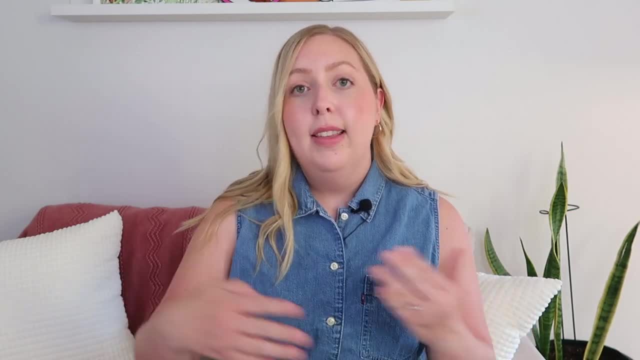 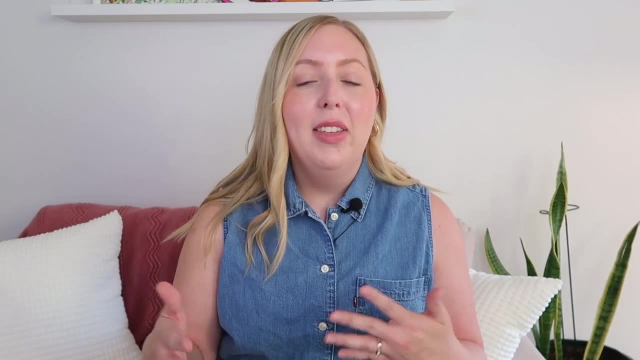 had a really fun time and it sparked some conversation. It was really nice, Like as they were moving they would talk to their neighbor about like oh, I really love Mario Grande. or like, oh, I can't stand her Right. So they could really talk about that musical. 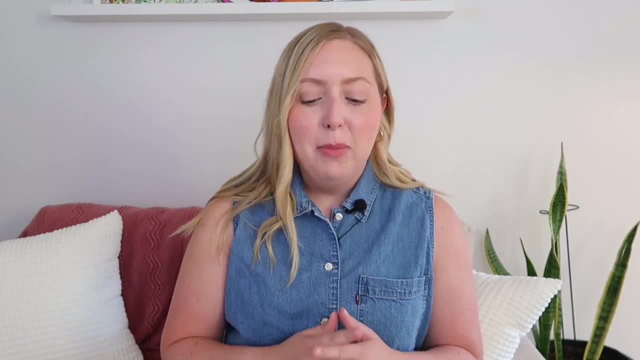 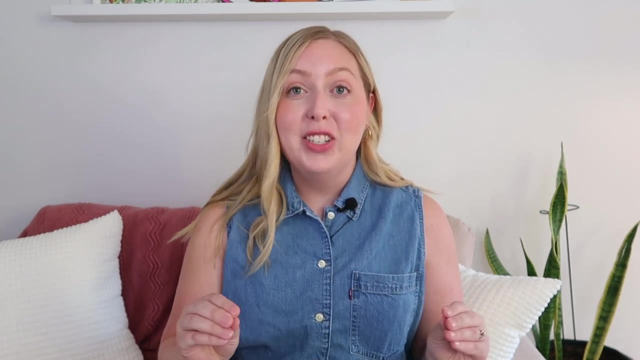 background and it just got the conversation going. So musicians move, Musicians move, It's also musicians. It's hard to say, So it was kind of funny. I mean, everyone try and say musicians. Side note, Okay, Anyways. second is: 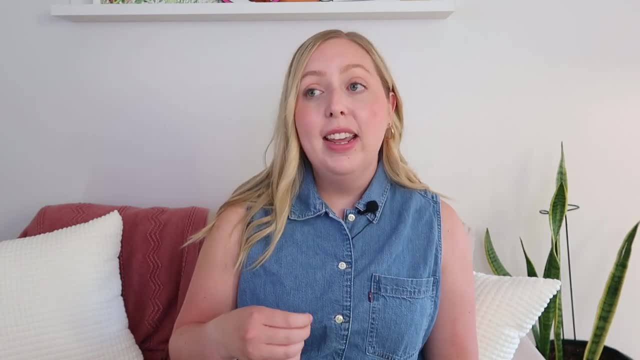 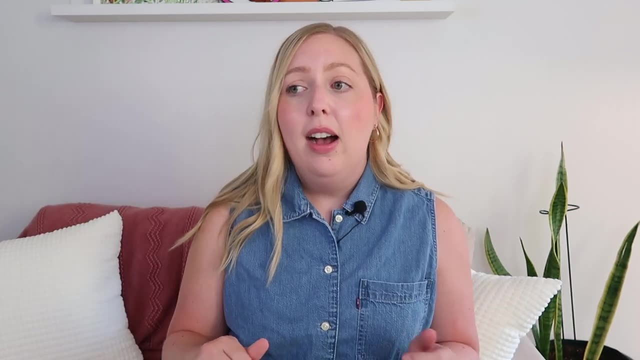 some quick rhythm review games. So I have an emoji game. I will put a picture of it here- and it's really simple. The students just pick an emoji, We click on it and we clap and say the rhythm They really like to get a kick out of just picking the emojis and seeing it. 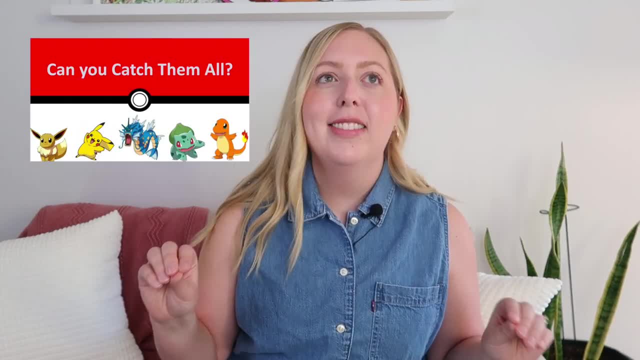 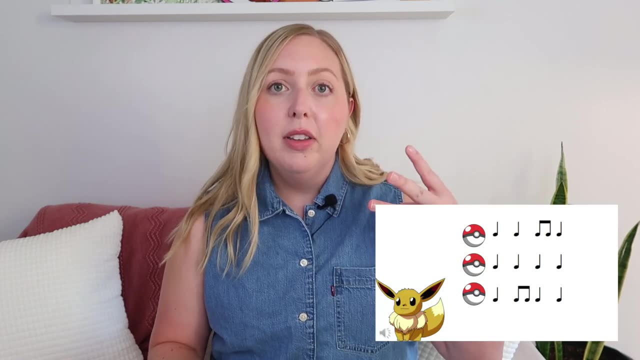 I also have a Pokemon game. I think that's a freebie, I'm pretty sure. Yes, It's in my freebie library and it's like got to catch them all. And so you pick a Pokemon and then you have three rhythms and I play one of them on rhythm sticks. The students have to identify the right one. 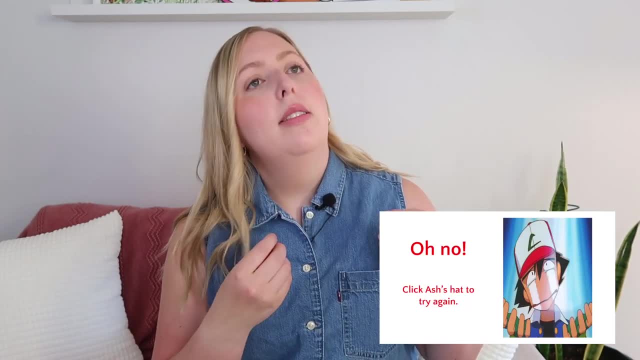 If they do, they get to pick one, And then I play one of them on rhythm sticks. The students have to catch the Pokemon, If not, it's like a crying face of Ash and he's like: oh man, you lost. 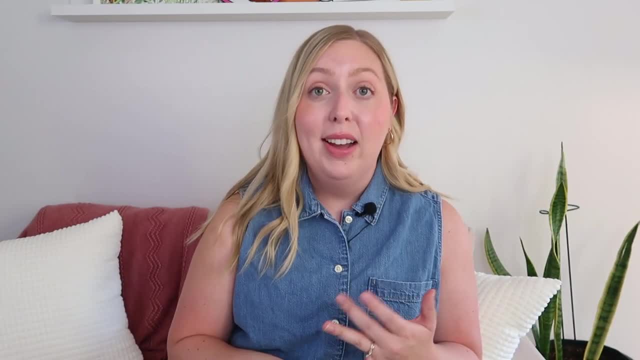 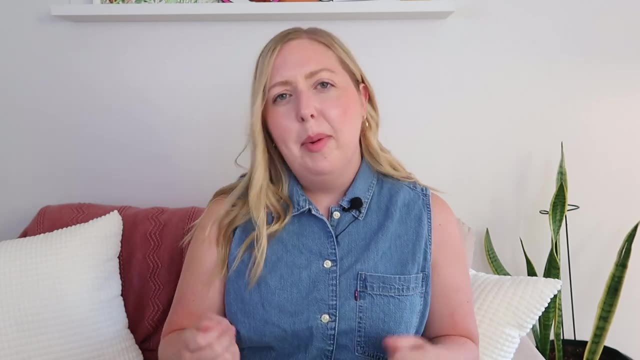 you didn't get it right And so you can just review that way. So just some fun review games. There's quite a few games like that out there and I think it just helps students kind of be like: oh yeah, I remember how to do rhythm. Third is these worksheets that I made. 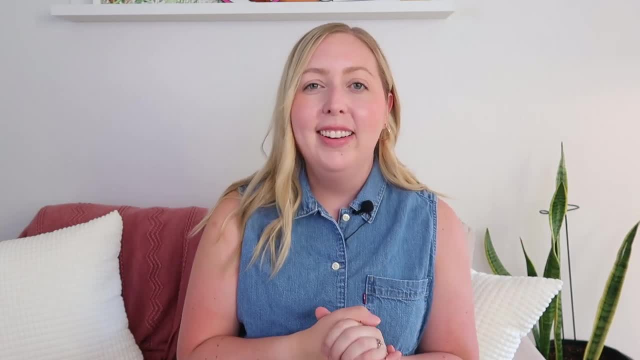 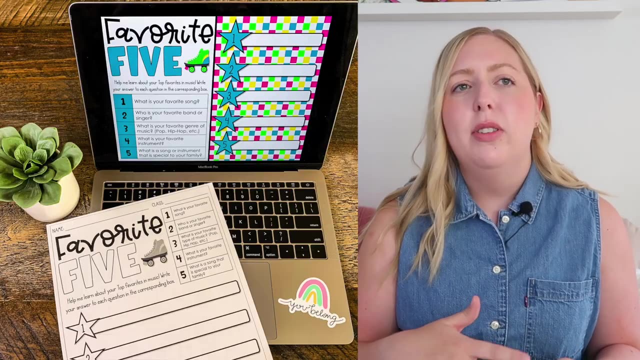 They're called First Day of Music Worksheets- What a creative title. And again it's helping you with your kind of getting to know their musical background. So I have things like your top five, And so you just pick one, And so you talk about your favorite song, your favorite artist, you know, so on and so forth. 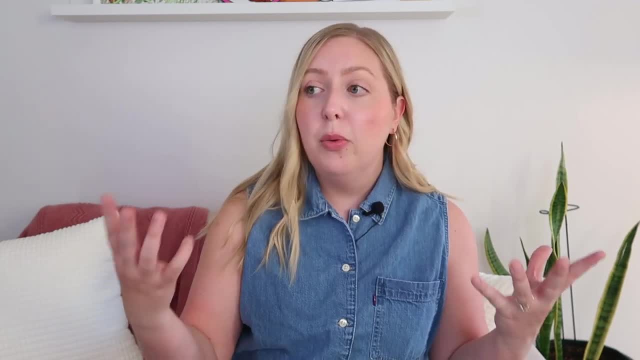 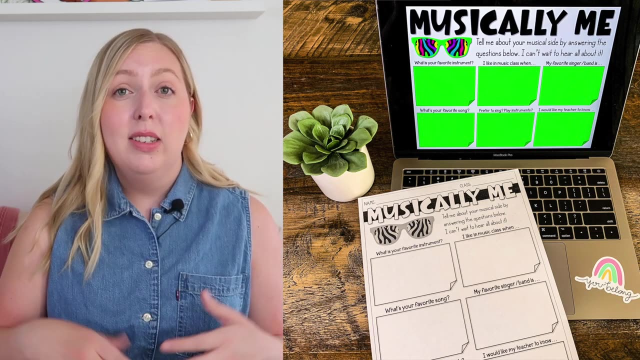 I have a like just a musical me one where they have a bunch of questions Kind of helps you. It talks about also, like you know, what do you like to do in music? What are you? a person that likes to be center stage? Do you like to sing? You know things like that just to kind of help you. 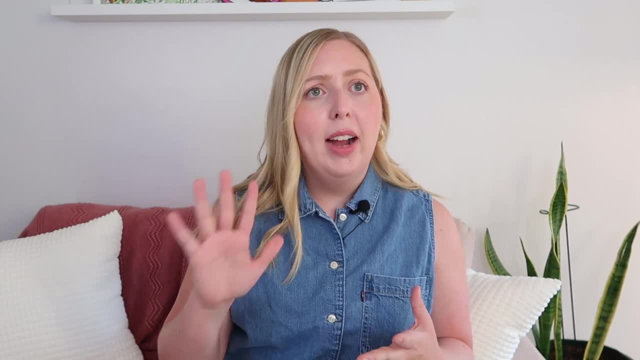 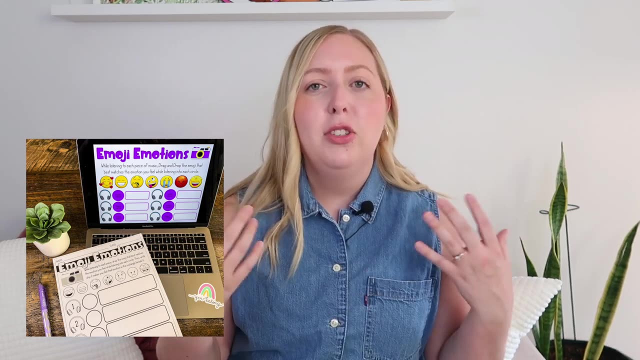 know a little bit more about them. So there's quite a few. I think there's five different worksheets in there. I think there's an emoji one where you listen to some music and you have to draw in the emoji that it made you feel, And so, again, it's just kind of a low pressure way to 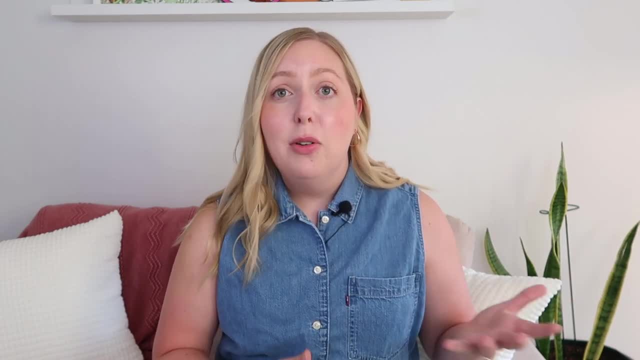 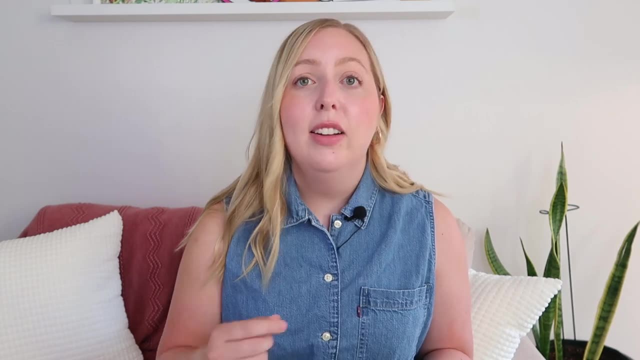 kind of get to know the students. That might be a great thing. Like you go through your procedures, kind of get through the seating chart and then you give them, you know, 15 minutes to complete this on their own. They can kind of chat with their neighbor while they're doing it. Really low key. 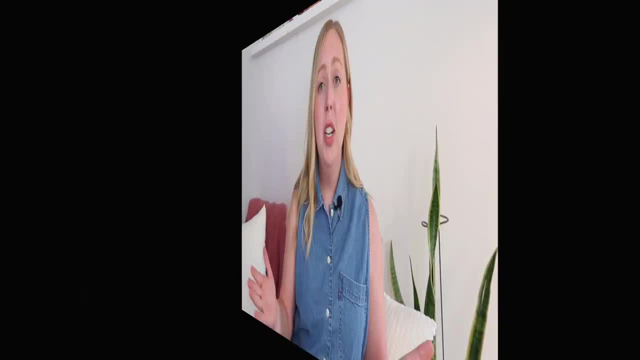 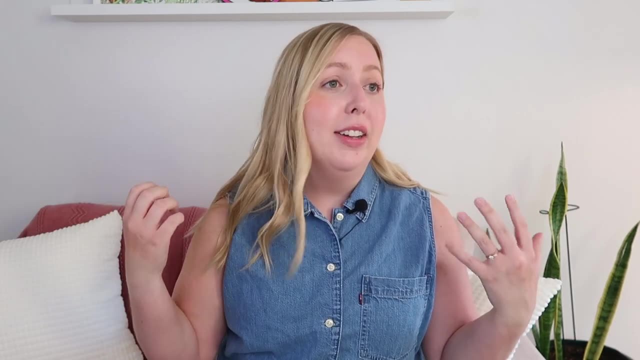 you know, good day for the first day of music, So let's talk about also instruments. I don't know about you guys, but as soon as my students come in, whether they're kindergarten or sixth grade, I get asked: when are we doing instruments? Like, that seems to be the most exciting thing to them. 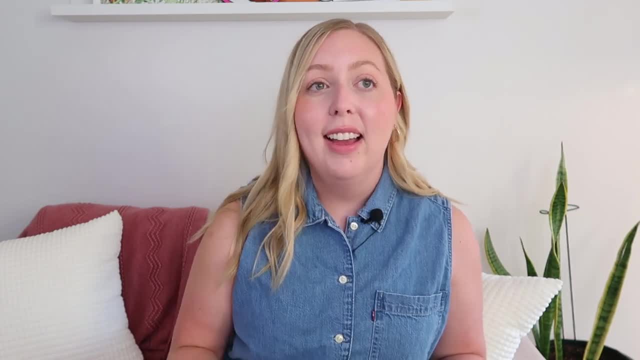 So a really easy instrument activity is called Yakety Yak. I have a link down below for you guys And it is to that song Yakety Yak. It's from, I think like the fifties, It's like an oldie. 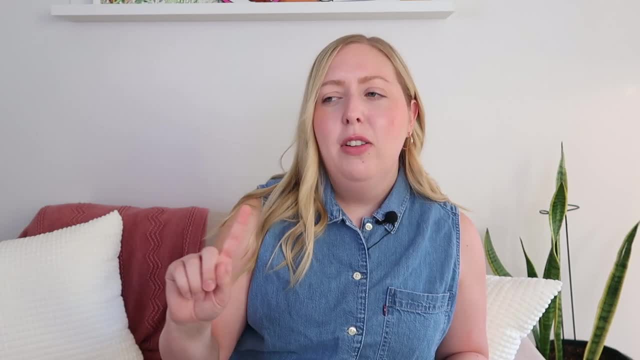 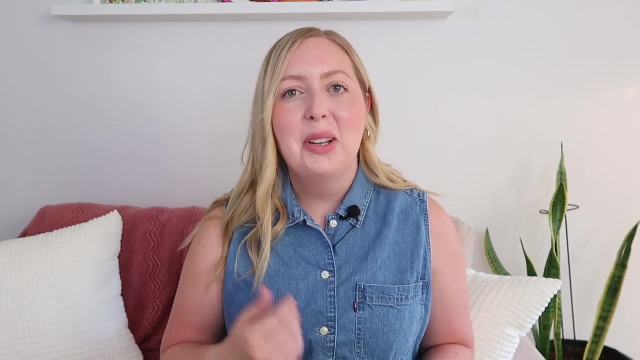 Take out the paper and the trash or you won't get no spending cash. Yakety Yak, don't talk back. Okay. So hopefully you got it from that. If you didn't, you can just look up the song. It's called: 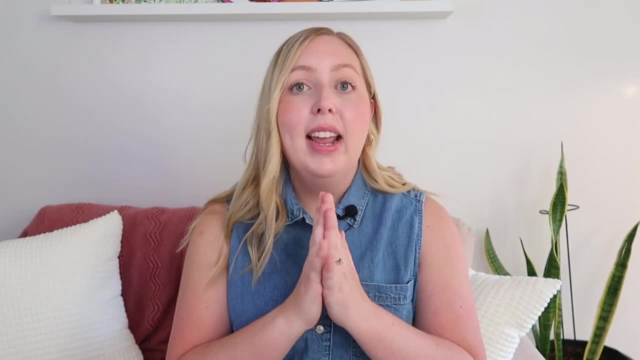 Yakety Yak. It's an oldie And it's like I just play it for them and I have them listen to it And they I say: okay, there's like a hidden meaning in this song. It's not literally a yak. 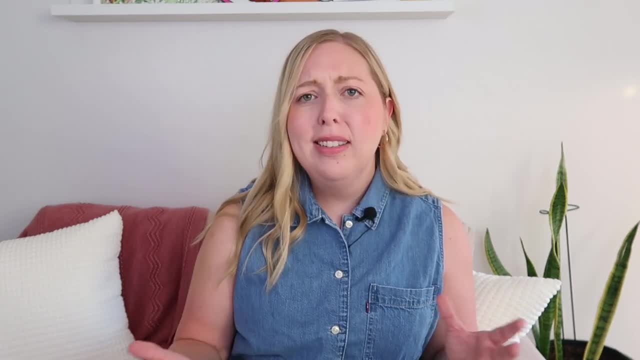 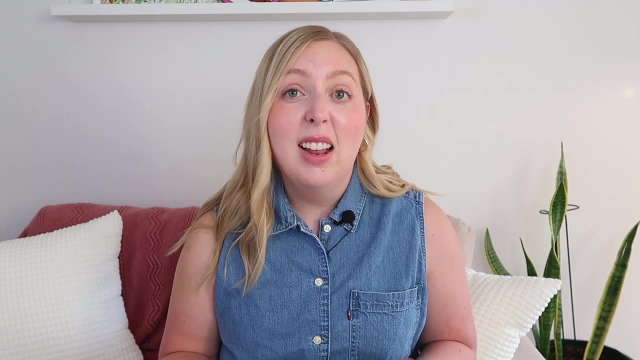 There's not a yak in the song. So I want you to listen and I want you to think about what does Yakety Yak mean, Or what's the story of this song? So I play it, they listen to it and you know, they start to pick up. oh it's. it's like a parent and a kid kind of talking about. 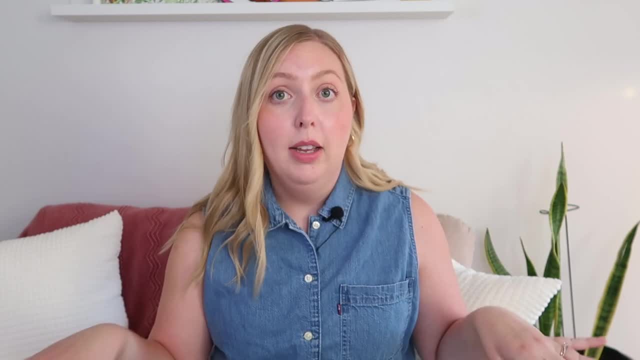 chores and the Yakety Yak means like: oh, whatever. like mom and dad or whoever right, I'm not whatever. Like they're not going to do this. like whatever right, i'm not whatever. like they're giving sass back to their, their parents. they're like i'm not. 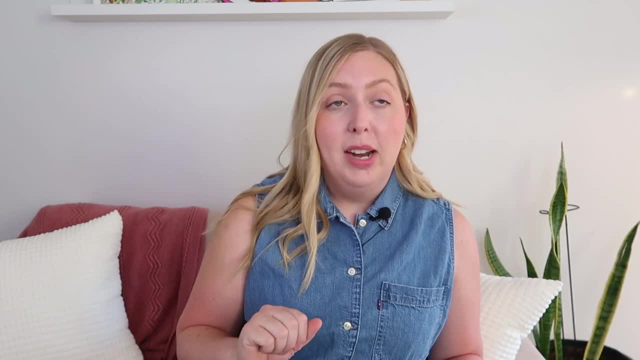 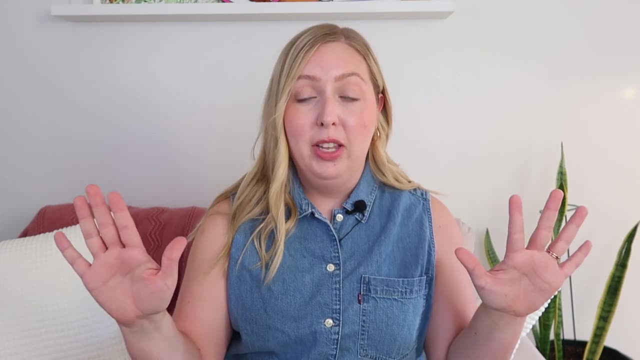 doing my chores and then don't talk back the parents like, oh, you're in trouble, right? so i'd say it's a kind of silly song about that relationship. once we get that, then i show them the image and i have an a section and a b section, and so the a section is gonna it's gonna be a. 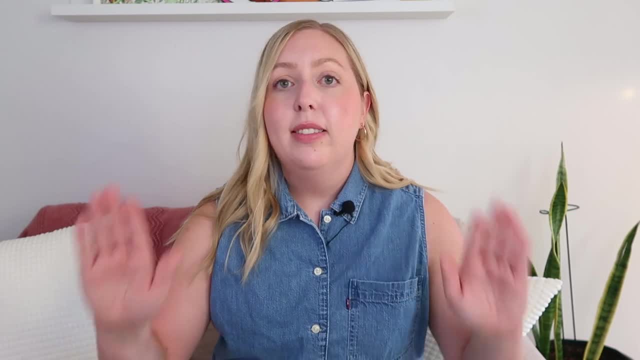 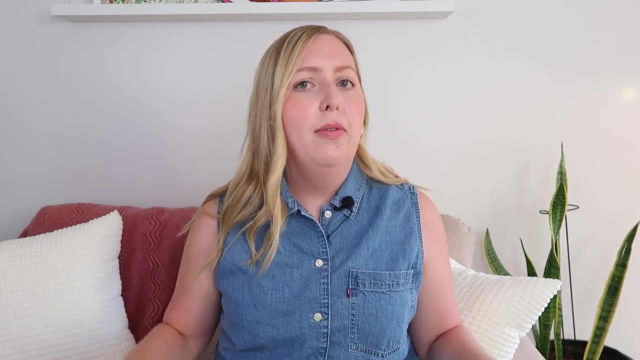 rhythm stick activity, and so i first just have them practice without rhythm sticks. i say, okay, pretend this your rhythm sticks, and it's out: two, three, four, five, six, seven, eight. the floor: two, three, four, five, six, seven, eight. your shoulders: two, three, four, five, six, seven, eight. and then here's: 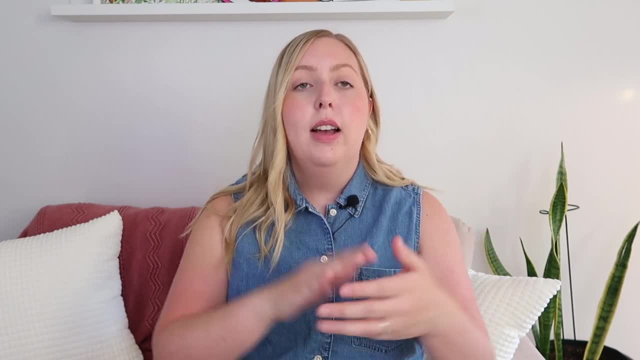 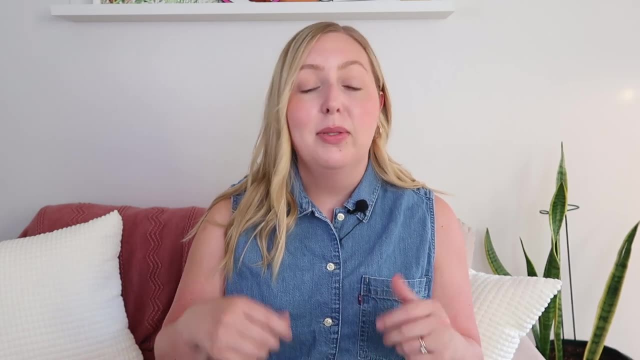 where it's like we have to do some practicing- out knees, shoulders- t t ta, rest, okay, and so that repeats and we talk about, you know, the out knee shoulders- t t ta, rest, rest, rest, rest- is where we really do have to practice. we practice that a few times. we talk about what the repeat sign is you. 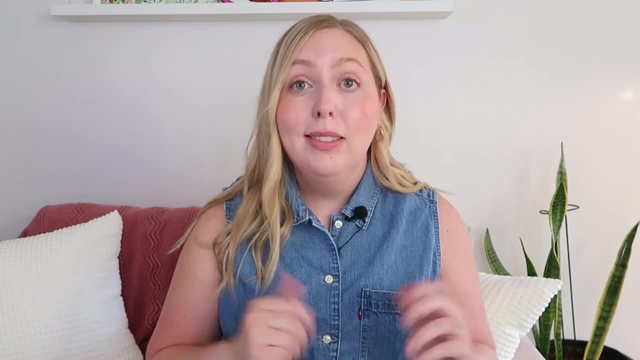 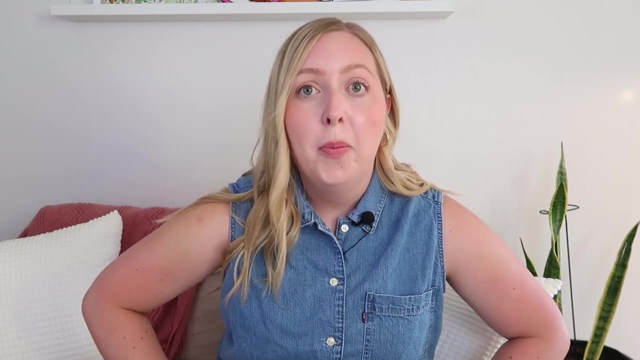 have to repeat it three times and then we go on to the b section. i say, okay, this is your time for fifth, sixth graders. this is only t, t, ta and rest. come on, we could do this. and i say, okay, go. and they try and clap the b section and it's a really good time just to kind of see what do we. 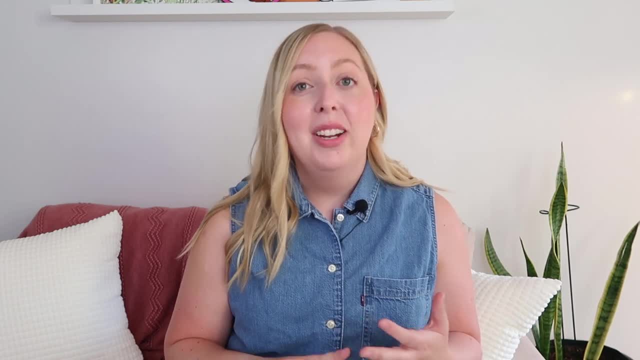 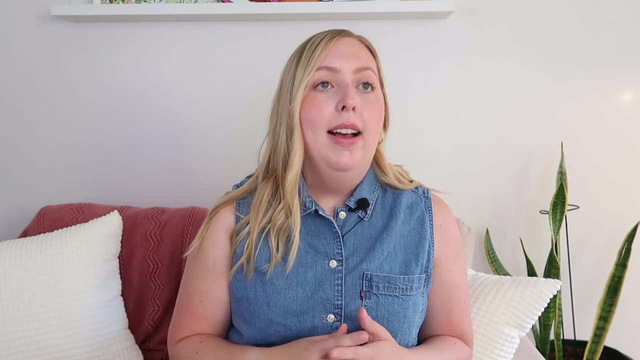 remember um, and usually by like the third line. that's where it gets a little messy. so we kind of go back and practice. we talk about, you know, showing the breast instead of saying or rest um, and things like that. so it gets a good, good little rhythm review right in there. 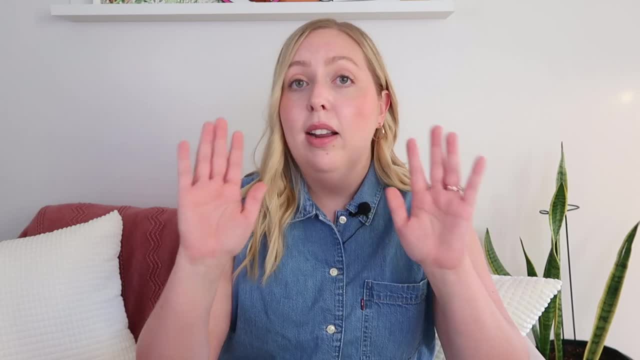 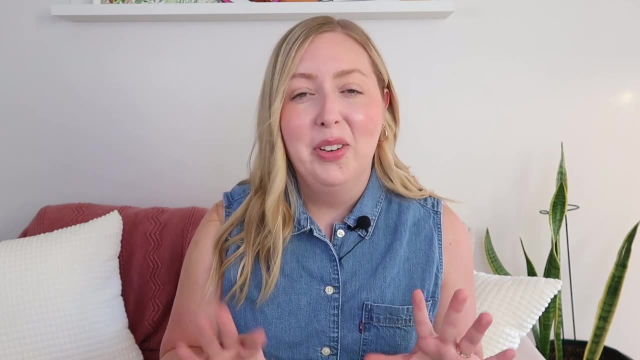 and then after that we practice it with the song, and so i put the song on and we just do air motions and clapping and then i get them paired up. i've been picking partners a lot more before. i used to let students pick partners a lot and i have just found it leads to a lot. 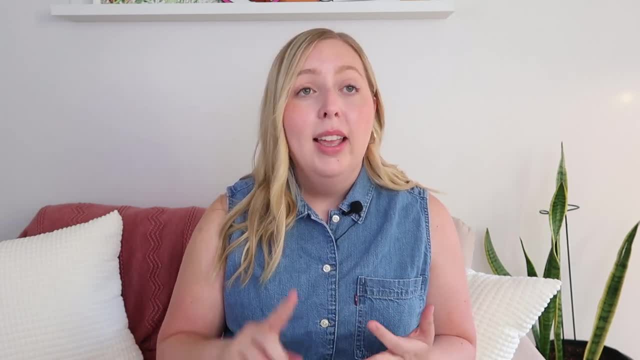 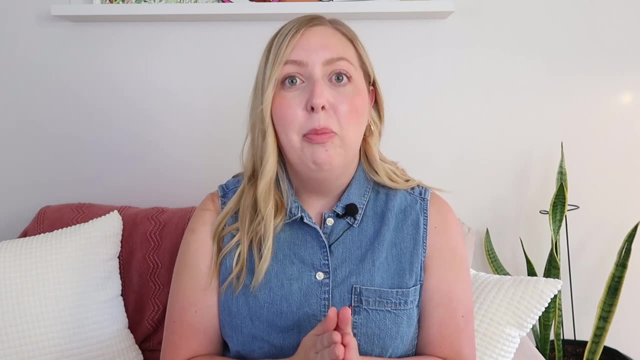 of anxiety. it leads to a lot of people being feeling left out, and so this year i'm just doing more of like i'm picking partners or i'm picking it randomly somehow, and so i think that's really helping. anyways, i pick partners and then they get rhythm sticks, and so 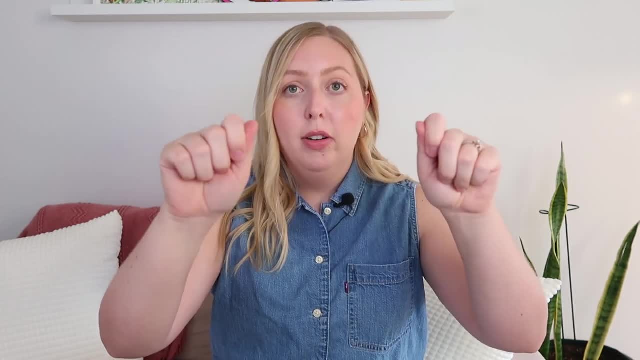 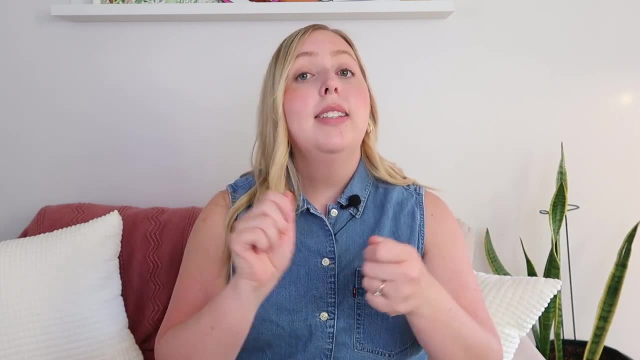 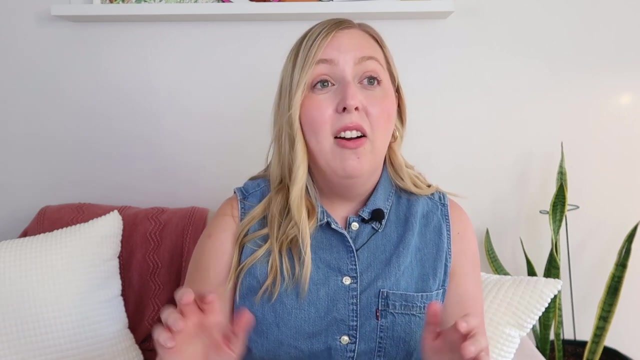 so now it's tapping out, is tapping your rhythm stick with your partner out eight times, and then the floor eight times shoulders. you're just tapping on your shoulders, okay, out, knees, shoulders, and then ti-ti-ta is to yourself. so ti-ti-ta, then I tell them: okay, you guys our rhythm sticks have. 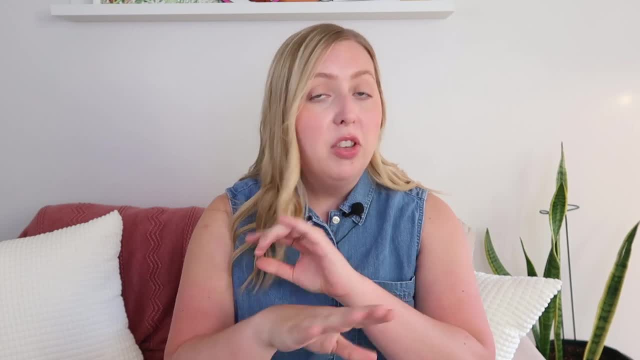 a bumpy side and a smooth side. so on the B section you need to play that rhythm. but you can play it however you want. you could scrape it, ti-ti-ta, ti-ti-ta, ti-ti-ti-ti-ti-ta. you can play it on. 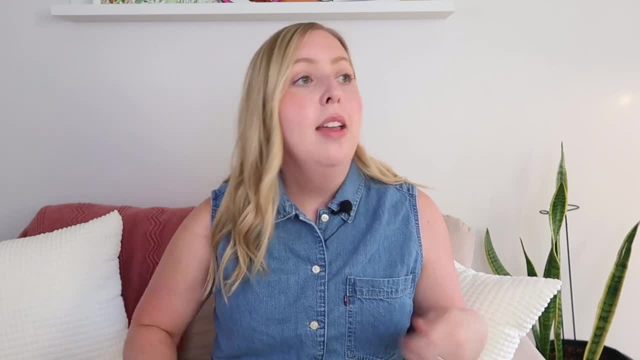 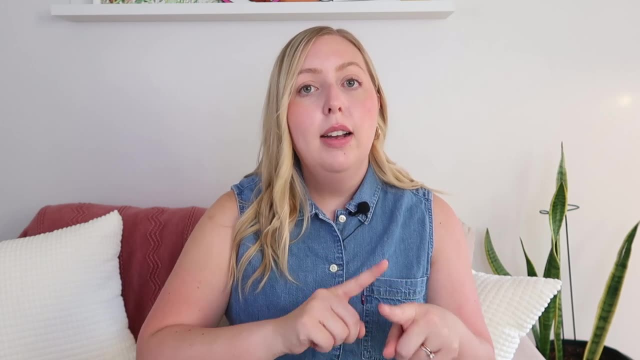 the ground: ti-ti-ta, ti-ti-ta, more of a drummer way. okay, you could play a combination. you could just tap it like this for tas and scrape for ti-ti-ti-ti-ta, ti-ti-ta, ti-ti-ti-ti-ti-ta, and so. 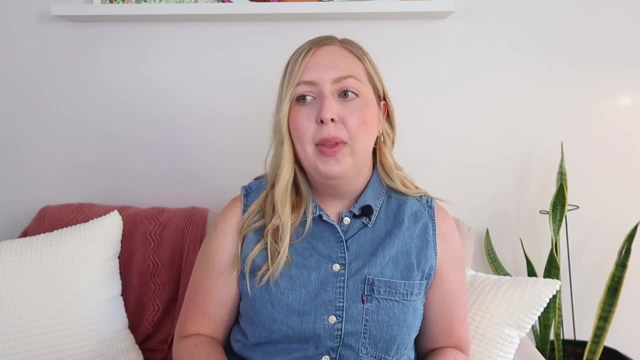 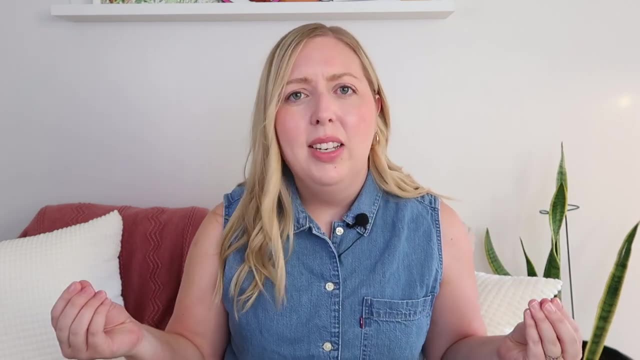 I give them a little bit of freedom and choice and how they play that rhythm, because then by then they're like we know this is too easy for us and I'm like: okay, well, then you play it some different ways and use your creativity. then we do the whole thing. it's a great time. 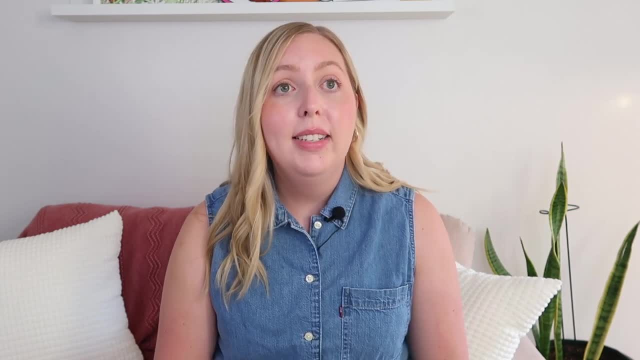 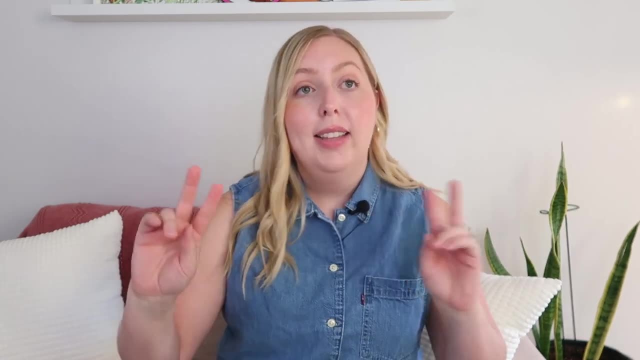 you and we wrap it up. so that is a really great first day or first two days activity. what I did is I split it up. so the first day we just did it with hand motions and then the second day we actually put it to music with the rhythm sticks. so four lesson ideas for your very first day with your. 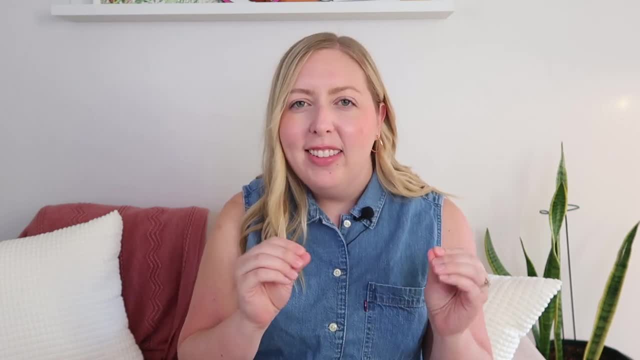 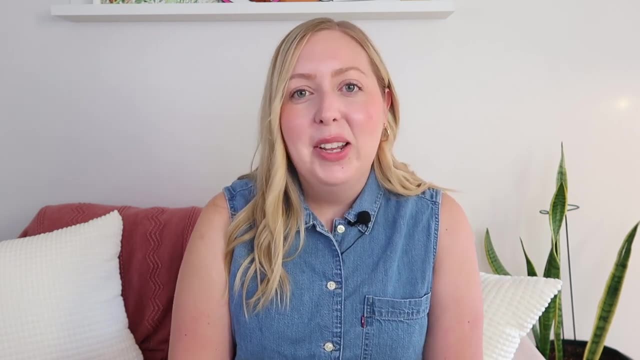 fourth, fifth or sixth graders. I hope that helped. hopefully there's something in there that you haven't heard yet, and I hope you have a great first day of music, whether it's happened already or it's to come, and I'll catch you guys in the next video. bye. you.